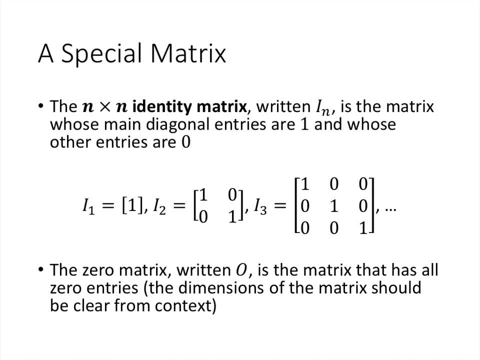 special matrices I want to talk about. The first is the n by n identity matrix. So that's a square matrix because it's got the same number of rows as columns, And this matrix has ones on that main diagonal that we were just talking about and zeroes everywhere else. So I1, that's. 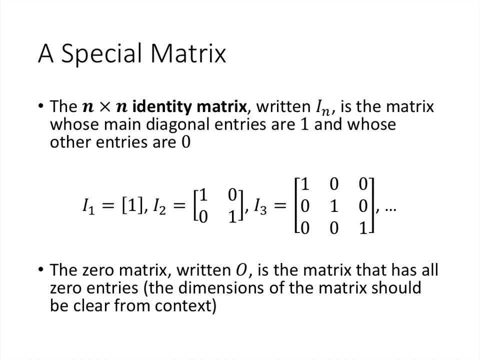 a one-by-one matrix with a one on the main diagonal. there's only the one entry there. I2 is a two-by-two matrix with ones on the main diagonal and zeroes everywhere else. I3 is a three-by-three matrix with ones. 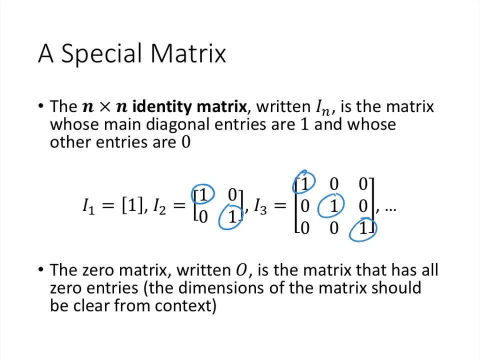 on the main diagonal and zeros everywhere else, and so on. Another special matrix that will come up occasionally is what we call the zero matrix, and that's just the matrix that has zeros for all of its entries. Now notice that that notation here, which is a capital O, doesn't indicate the size of 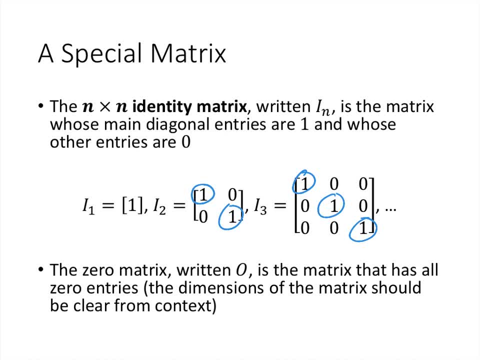 that matrix, but usually that size will be clear from context. Something else that you may sometimes see is you may see the zero matrix written as a number zero. I find that notation confusing because obviously zero already has a meaning as it's just a number by itself. so I'll typically write the 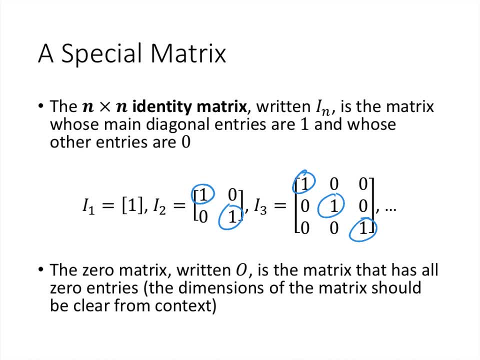 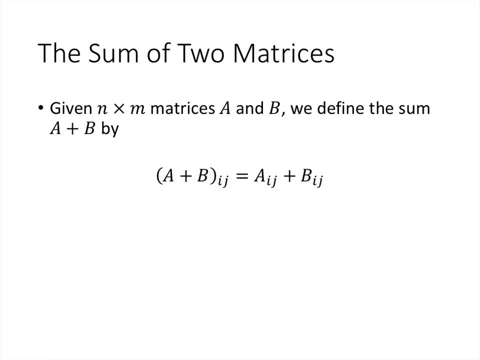 capital O, but you may see the number zero used for this matrix as well. Now we can start defining operations on matrices. So the sum of two matrices if they have the same size, so they both have to have n rows and m columns, but the definition is that the sum of 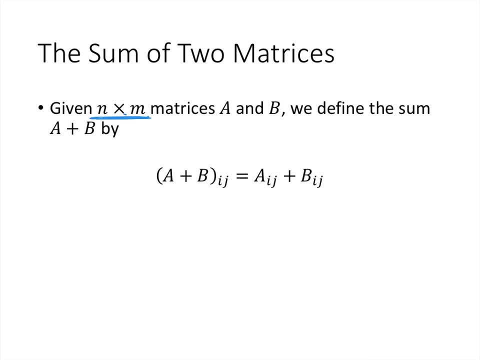 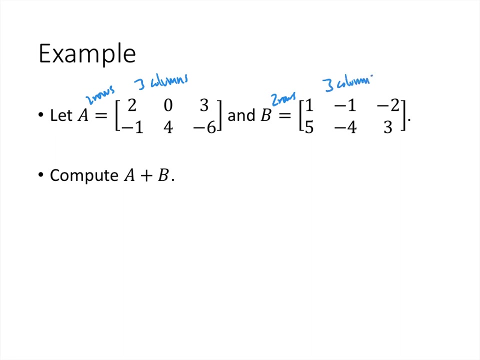 those two matrices is performed entry-wise, So the ij entry of a plus b is the ij entry of a plus the ij entry of b. So, for example, here we have two matrices that are the same size. They both have two rows and three columns, and so that means that we can add them together. 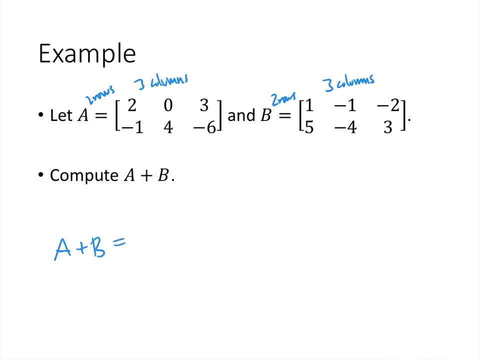 And the way that we add them together is we just add the corresponding entries together. So the row one column one entry of the sum of these two matrices is the row one column one entry of a plus the row one column one entry of b. 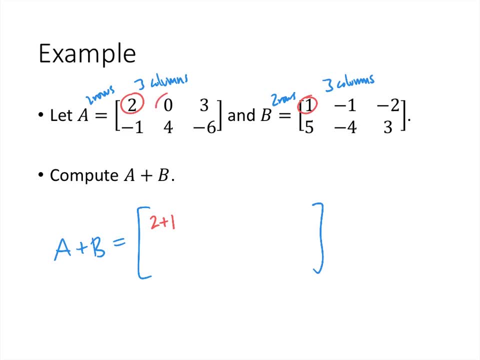 So that's just going to be two plus one. The row one, column two, entry is going to be the sum of the row one, column two entries. so that's just going to be zero plus negative one, And then we continue in the same way. So three plus negative, two negative one plus five. 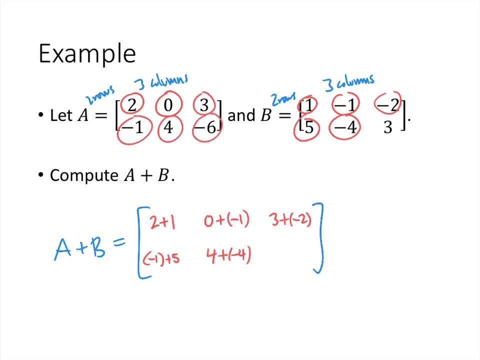 four plus negative four and negative six plus three, And so when we do all those additions we get three negative one, one, four, zero negative three, And that would be the sum of these two matrices. Another operation that we can do is to multiply a matrix by a scalar, And again: 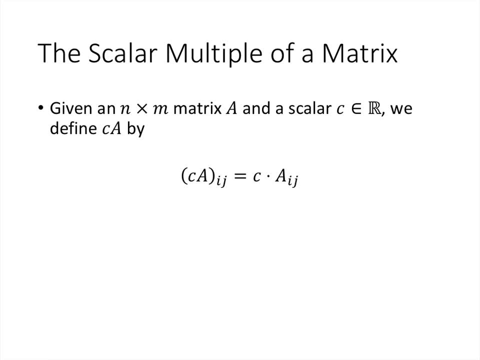 this is pretty straightforward: All we're going to do is multiply each entry of the matrix by that scalar. So, for example, here we have a matrix A and if we want to define three times A, all we're going to do is multiply each entry by three. So three times two, three times zero. 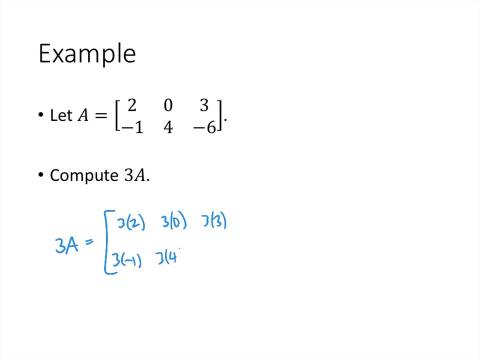 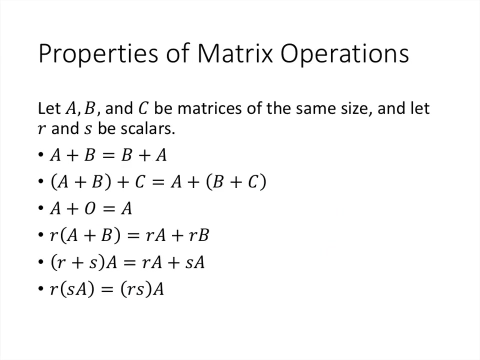 three times three, three times negative one, three times four and three times negative six. And we do all those products. we get six, zero, nine negative three, twelve negative eighteen. Pretty straightforward. Now, with these operations under our belt, we actually have some nice properties that. the operations satisfy. The first property here is that we have a decrease in the number of approaches. You don't have to calculate by doing less than one operation. You can just spend the test values and the rest of the time, and the results are just an estimate of what the one operation is getting. 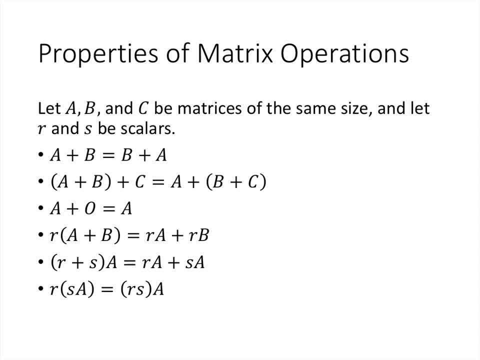 And that's how we get things we want to get. So if we do the specified expression in order to look at the empty groups, it's the first operation that you can see. The first property here is that the addition operation is commutative. 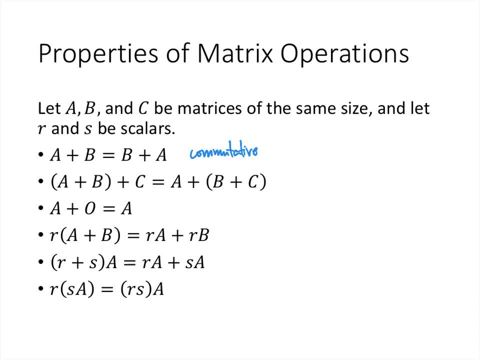 So the order in which we perform the operation doesn't matter: A plus B, B plus A- same thing. The second nice property that we have is that matrix addition is associative. The grouping doesn't matter If we have A plus B plus C, it doesn't matter if we do the A plus B and then add the C. 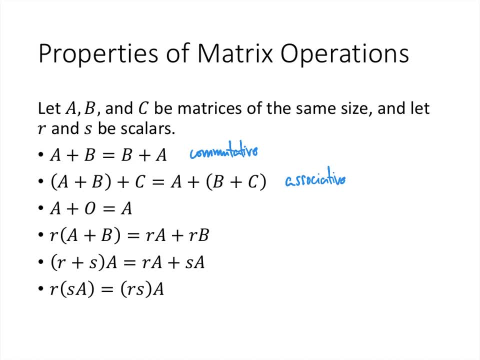 versus if we do the B plus C and then add the A. The third property here is that we have an additive identity. The matrix O is the additive identity here, because adding it doesn't do anything to the matrix A. The next two properties are distributive properties. 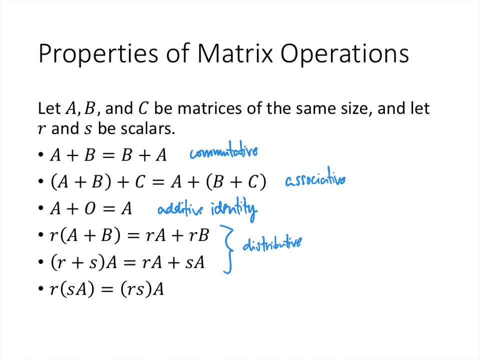 Multiplying the sum of two matrices by a scalar, we get distributivity. so we can multiply by the scalar individually, and that's the same if we add the two scalars and then multiply by the scalar And the last property. here is a kind of associativity. 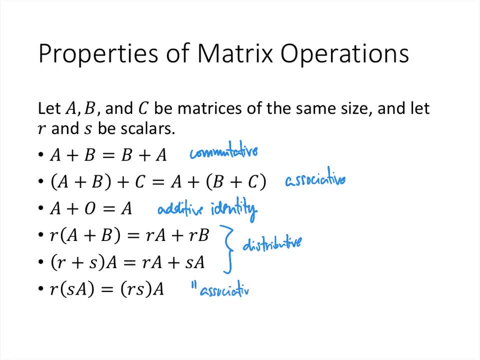 I'm going to write associativity in quotation marks here, because it's not really quite associativity, because it's not the same operation in each of the sets of parentheses. This R times S. that's just multiplication of two real numbers. That's just multiplication in the set of real numbers. 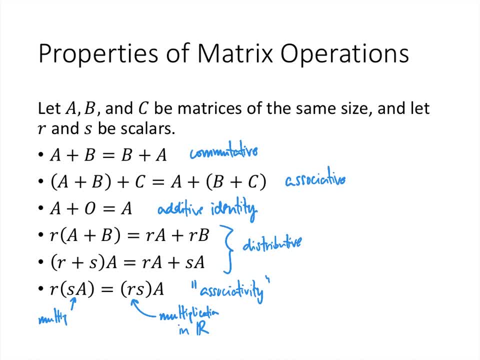 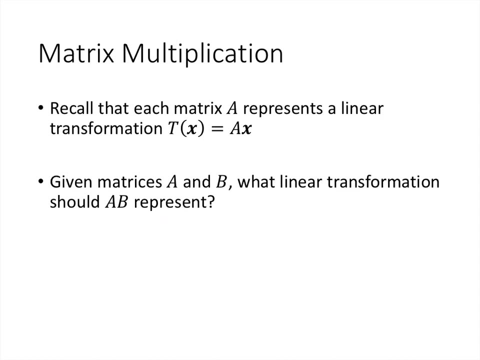 But S times A. here that's multiplying a matrix by a scalar, So it's not really quite the same thing, But it looks like associativity. It has the same visual sense that makes us think of associativity. All right, now we're ready to talk about matrix multiplication. 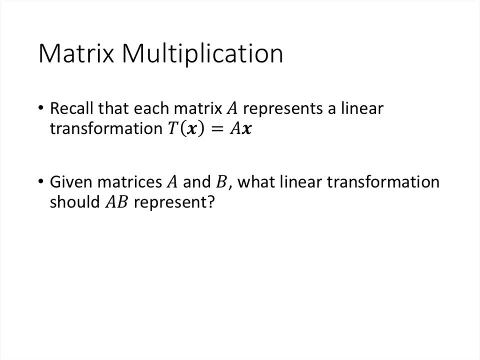 So this is a slightly more complicated operation, and the motivation here is that we want to remember that each matrix represents a linear transformation. So we can define a linear transformation using the matrix A by simply defining T of X to be A times X. So, given matrices A and B, 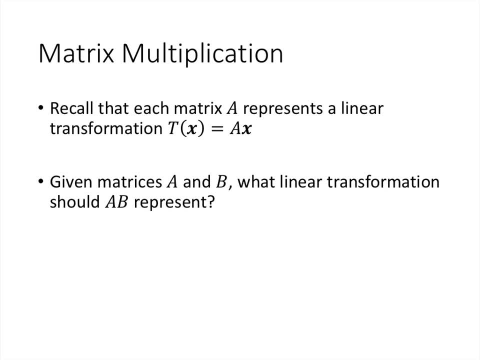 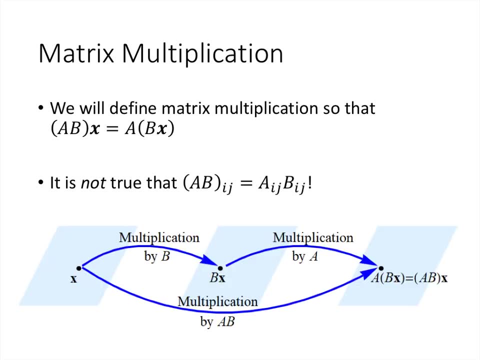 which represent their own individual linear transformations. what linear transformation should the product of those two matrices represent? Well, here's the idea. We want to represent, A times B, the matrix A times the matrix B, by the composition of those two operations. 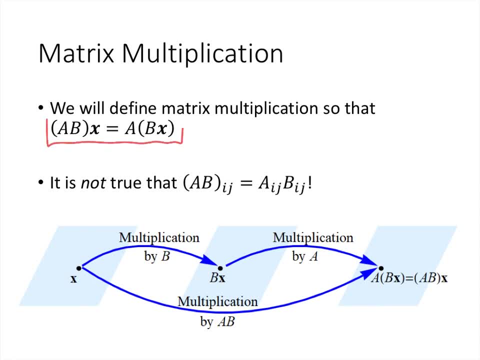 So in other words, we want this equation ABX equals ABX to be the defining property for matrix multiplication, And it's going to turn out that we're not just going to multiply the entries of A by the entries of B, like we did for addition. 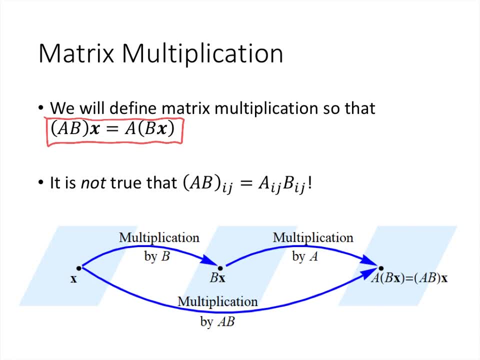 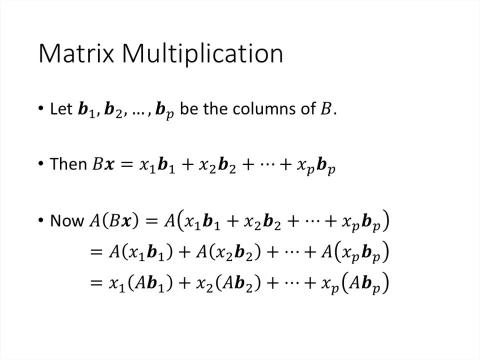 It's going to end up having to be a little bit more complicated. So here's how we're going to derive our matrix multiplication rule. We're going to give names to the columns of capital B, So little b1, little b2, and so on. those are the columns of B. 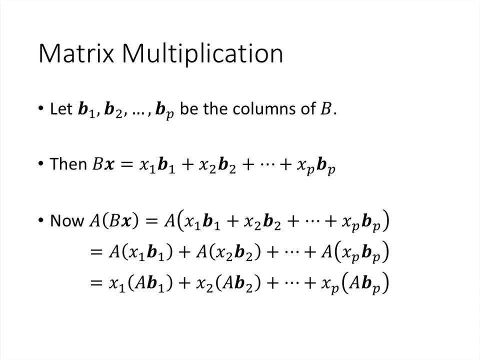 So that capital B times X. as we know, multiplying a matrix by a vector just gives us a linear combination of the columns of that matrix. So if the X1 and X2 and so on are the entries of the vector, X, X1 times b1 plus X2 times b2,. 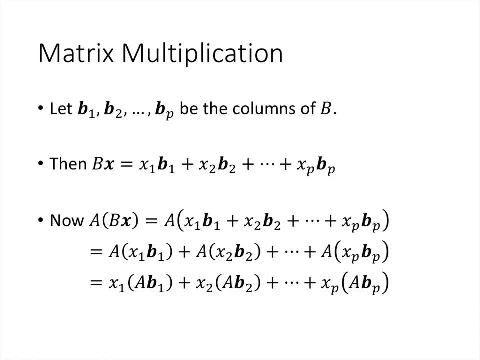 that's what it means to multiply the matrix capital B times the vector X. So now we're going to multiply this BX by A, And so all we've done here is take this expression for BX and substitute it in for BX in this next equation. 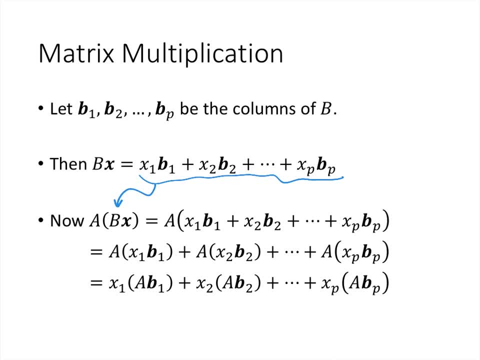 And now we're using algebraic properties of matrices multiplied by vectors. This is a distributive property, which lets us distribute the multiplication by A across all the individual vectors. And then another one of our properties that we have is that we can take scalars, and each of the individual Xs is a scalar. 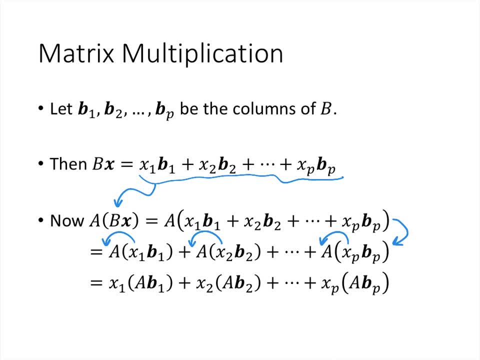 and move it outside the multiplication. So we have this X1 times AB1,, X2 times AB2, and so on. And what I want you to notice here is that this last line is a linear combination of the vectors AB1,, AB2, and so on up through ABP. 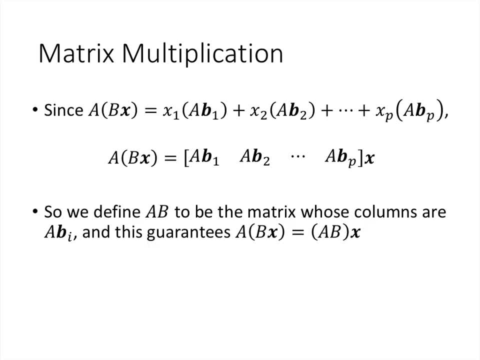 And remember that we can represent linear combinations of vectors as a matrix times a vector, where the scalars of the linear combination are the entries of the vector and the vectors that we're finding the linear combination of. those are the columns of the matrix. 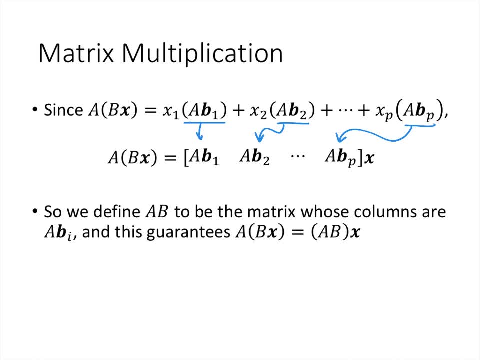 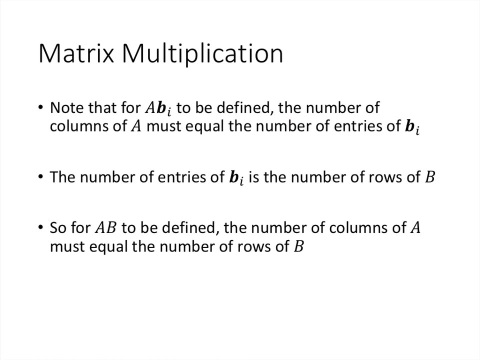 And so what we have here is our definition of our matrix AB. So this matrix here, whose columns are the capital A times the little b's, that's our definition of capital A times capital B. Now there's an important note here, In order for this to make any sense. 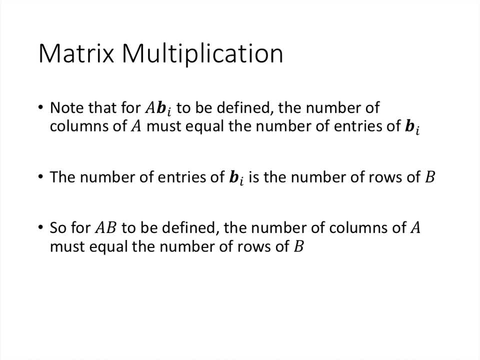 in order for capital A times little b i to be defined, any matrix times any vector. for that to be defined, the number of columns of the matrix has to equal the number of entries of the vector, And so that means that the number of columns of the matrix capital A. 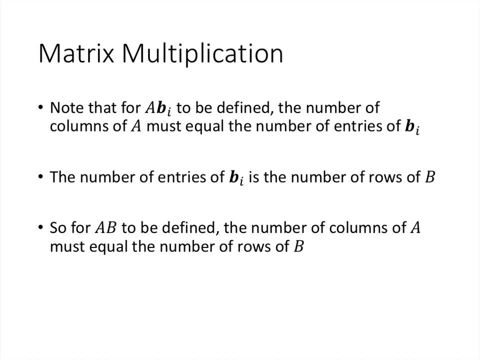 has to equal the number of rows of the matrix capital B. If those two numbers don't match up, then the product capital A times capital B is not defined. So let's carefully work through an example. In this case we've got a matrix A. 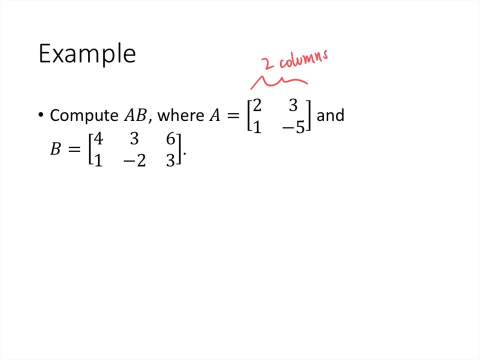 which has two columns, and a matrix B, which has two rows, And since those numbers match up, that means that the product A times B will be defined, And the way that we defined that is that A times B the columns of that matrix. 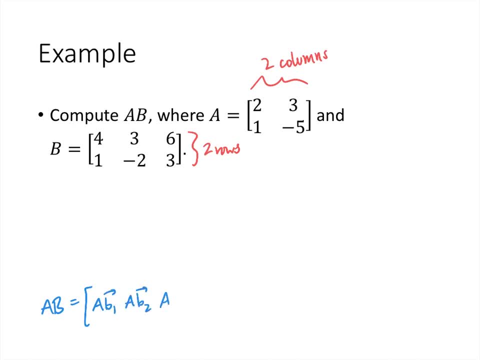 are going to be the matrix capital A times each of the individual columns of the matrix capital B. Since B has three columns- there's B1,, there's B2, and there's B3,- our product matrix AB is also going to have three columns. 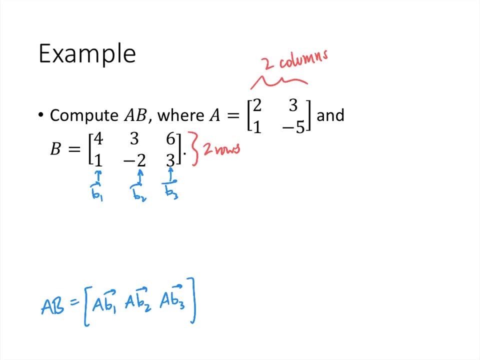 The matrix capital A multiplied by each of those columns of capital B. So all we need to do is figure out those columns individually. So A times B1, that's the matrix A, which is 2,, 3,, 1, negative 5,. 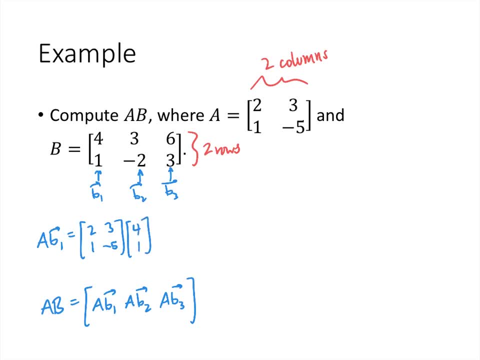 multiplied by the vector B1,, 4,, 1.. And then we have the matrix A, which is 2,, 3,, 1,, negative 5,, multiplied by the vector B1,, 4,, 1.. And then we have the matrix A, which is 2,, 3,, 1, negative 5,. 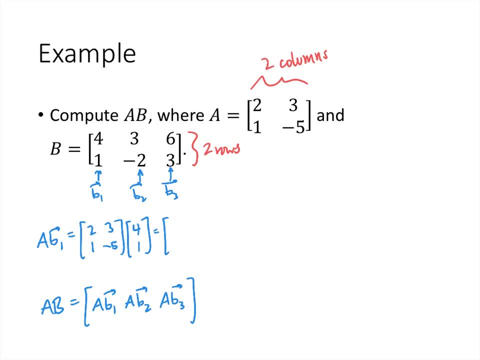 multiplied by the vector B1,, 4,, 1.. And now remember that we had a quick rule for multiplying a matrix by a vector: We go across the rows of the matrix and down the column of the vector, So we get 2 times 4, plus 3 times 1, that's 11.. 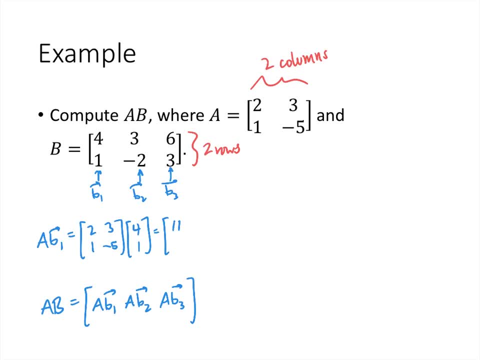 1 times 4, plus negative 5 times 1,, that's negative 1.. And so that vector becomes the first column of our product matrix. Next we figure out A times B2.. So that's the matrix: A, 2,, 3, 1, negative 5,. 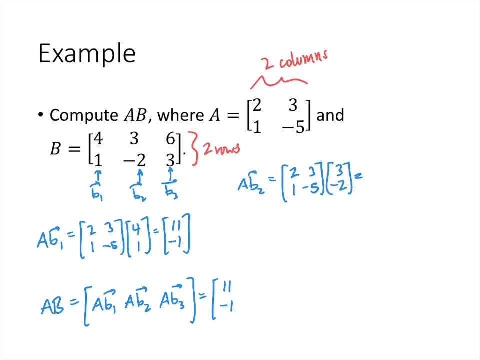 multiplied by the second column of the matrix, B, 3, negative, 2.. And again we go across the rows of the matrix and down the column of the vector. 2 times 3 is 6,. 3 times negative 2 is negative 6, add those together I get 0.. 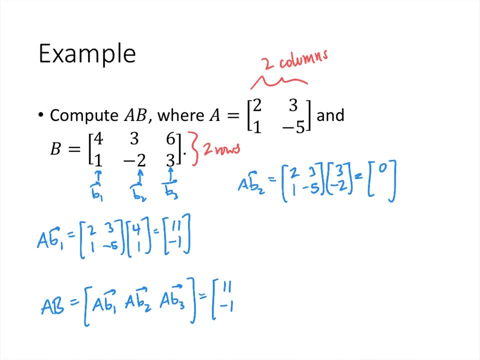 1 times 3 is 3, negative 5 times negative, 2 is positive 10, 3 plus 10 is 13. And so 0, 13,. that's the second column of our product matrix. Finally, we take A times B, 3, 2, 3, 1, negative, 5, multiplied by 6, 3.. 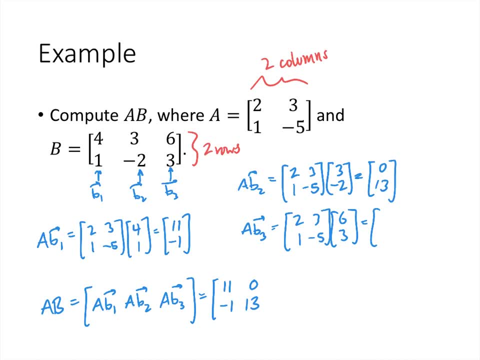 2 times 6 is 12,, 3 times 3 is 9,, 12 plus 9 is 21.. And then 1 times 6 is 6, negative. 5 times 3 is negative 15, add those together I get negative 9.. 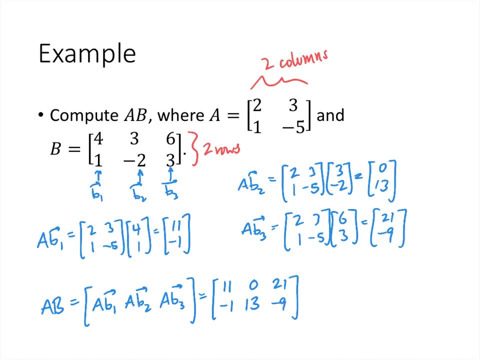 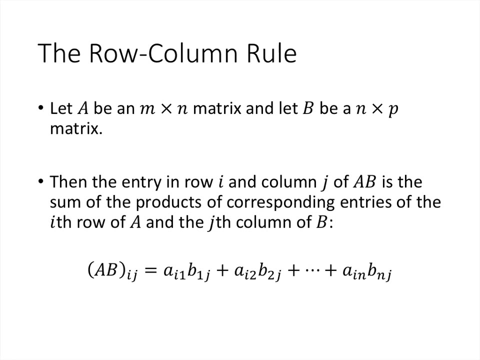 So 21, negative 9, that becomes the third column of my product matrix. So this, right here, that is capital A, Times capital B. Now this may seem a little tedious but we can piggyback on the quick rule that we had for multiplying a matrix by a vector.